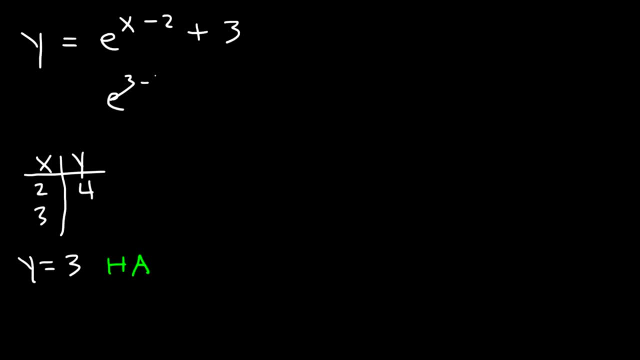 What is the value of y? So 3 minus 2 is 1.. e to the 1 is just e, And e is about 2.718.. But let's round it and say it's 2.7.. 2.7 plus 3 is about 5.7.. 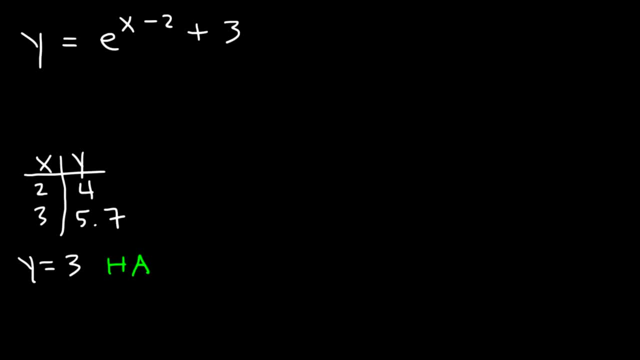 And now we have enough information to make the graph. So let's start with the horizontal asymptote at 3.. When x is 2, y is equal to 4.. When x is 3, y is going to be about 5.7.. 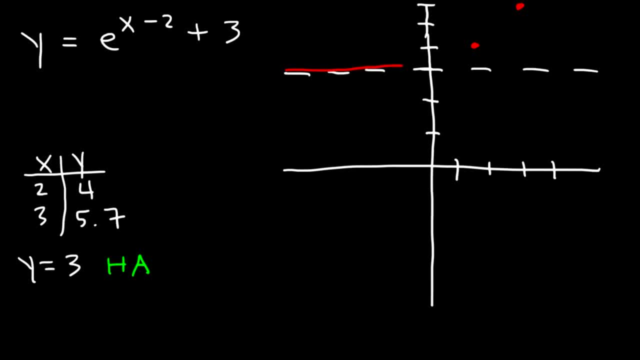 So very close to 6.. The graph is going to start from the x And it's going to follow the two points, So the domain is all real numbers, From negative infinity to infinity. The range is based on the y values. 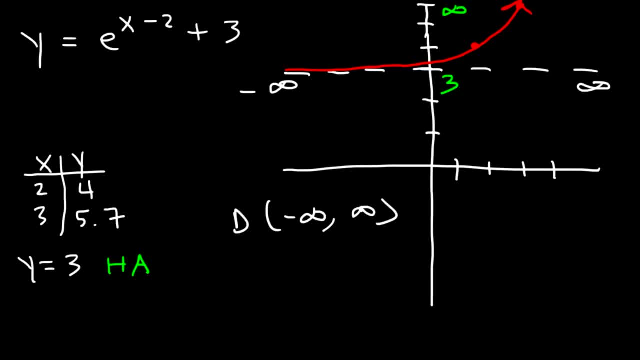 The lowest y value is 3.. The highest is infinity. So the range is from 3 to infinity. Now let's try an example with the natural law function. Let's say ln x minus 1 plus 2.. So this time we're going to set the inside part equal to three things. 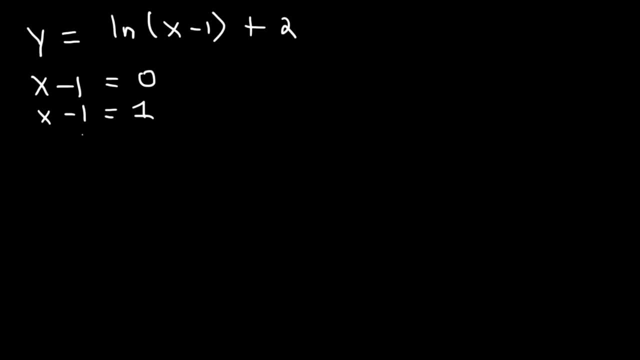 0,, 1, and whatever the base is, The base of a natural law function is always equal to e. And now let's find the value of x. So the first one where x equals 1,, that is the vertical asymptote. 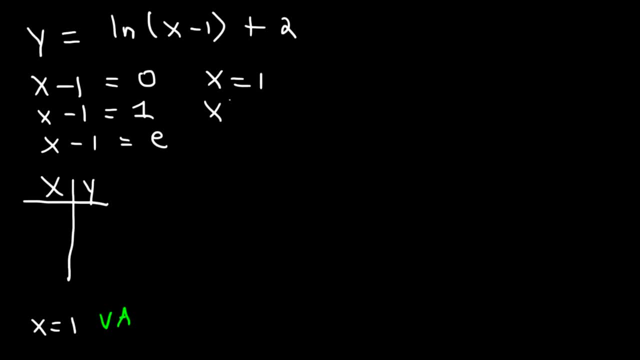 And when x minus 1 is equal to 1,, if you add one to both sides, 1 plus 1 is 2, so x is 2.. And if the other one is e plus 1, where e is 2.7.. 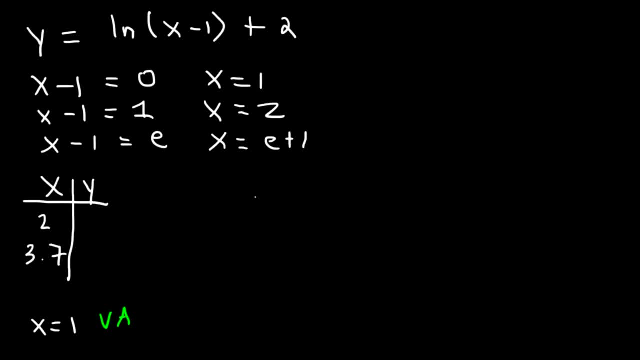 2.7 plus 1 is about 3.7.. So now let's find the y values. So let's plug in 2.. 2 minus 1 is 1.. ln 1 is 0.. 0 plus 2 is just 2..